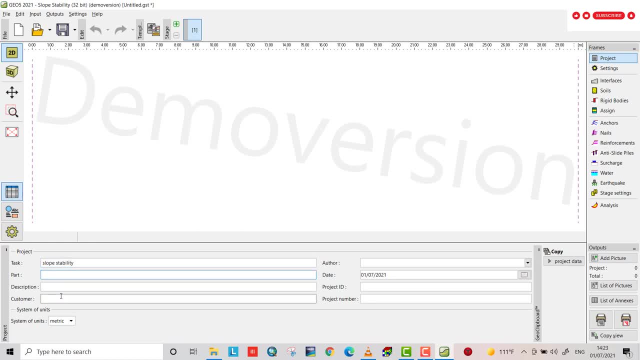 Part. also, you can provide part description, customer, for who you do the work and the system. I choose metric And I can provide some information about myself, my name, Rashad Mohammed, the date, project ID or project number. Okay, From settings you see earthquake analysis standard. 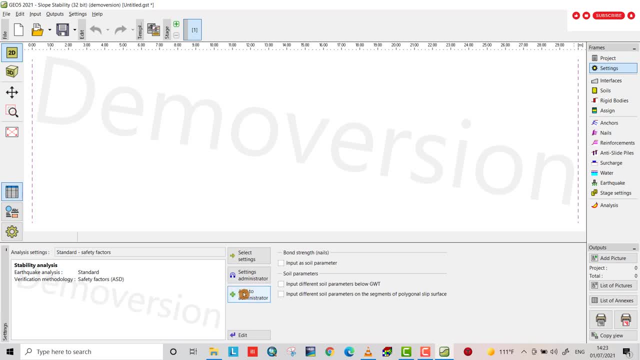 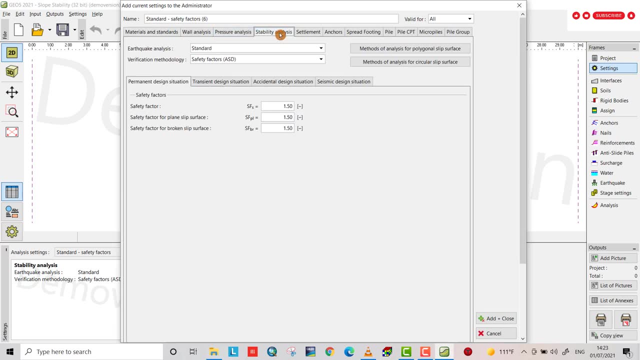 And verification methodology. safety factor Also, you can change the verification methodology from add to administrator And slope stability. Oh sorry, stability analysis, Earthquake analysis. you have different options. I choose standard. Also, from verification methodology, I have different options. 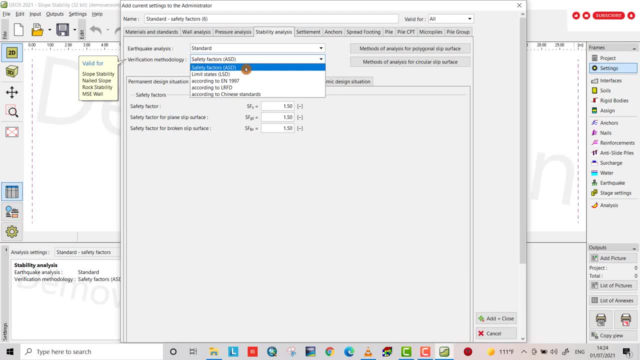 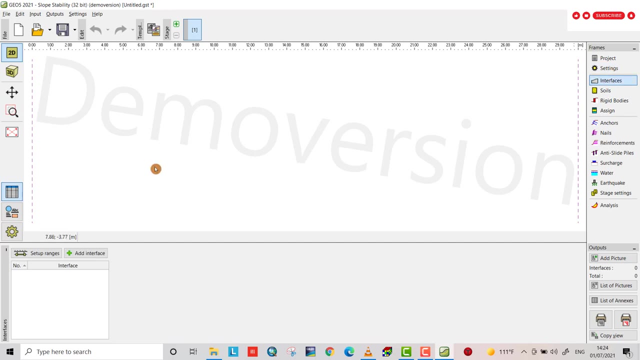 I choose safety factor And you can choose which one is your preferred. That's safety factor For safety factor 1.10.. Safety factor for planes with surface 1.5.. Also, you can change the safety factors. Okay, Interface. 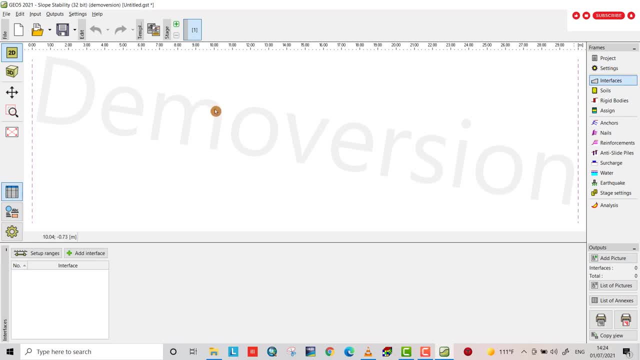 We have three methods to bring interface or make interface in the geofile. First, if you have the DXL file from AutoCAD or Cipher or any other drawing programs, Just save the drawing in DXL file and import to the geofile by template. 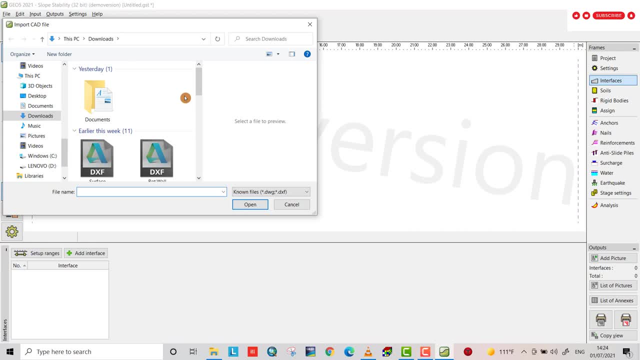 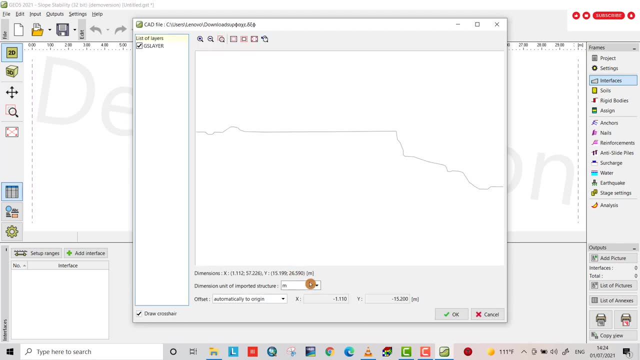 From template. Then select the file Surface. Okay, Here you have some options. Which is the unit, Unit meter You can change. I choose meter Automatically to origin. No, I choose no offset. When you choose no offset, you can bring different files and they fit together. 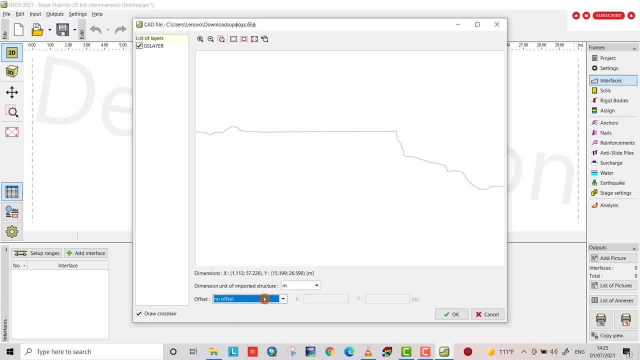 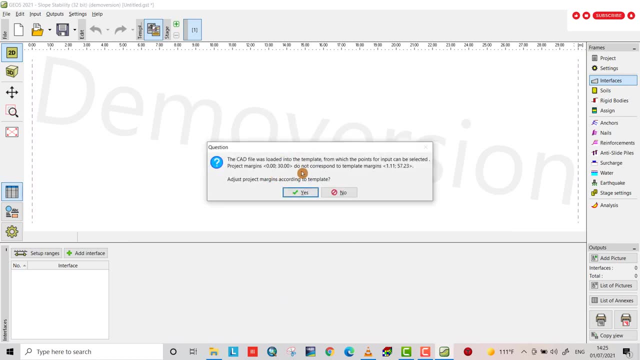 Otherwise it not be fit to Together So. So that's why I choose no offset. Okay, You see Project margin 0 to 30 and do not correspond to template margin 1.11 to 57.23.. 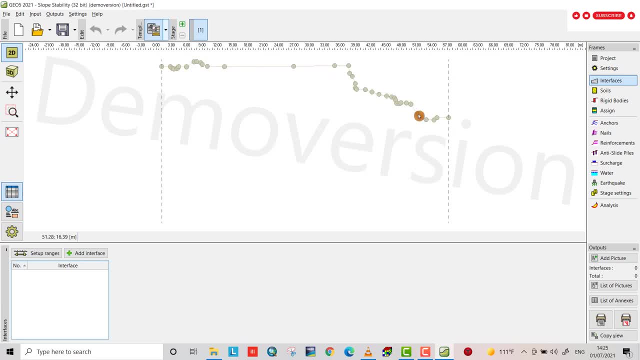 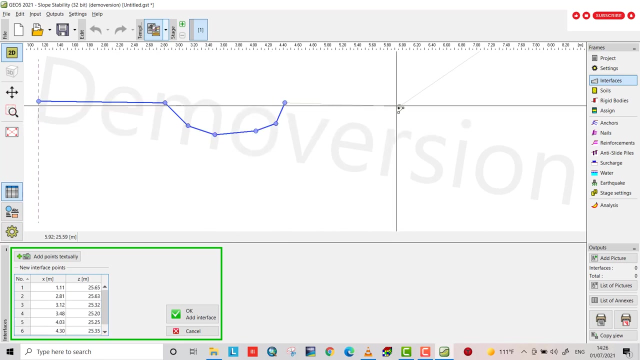 Adjust, Yes, Adjust, That's the point. We just draw the interface Through this point. we have Okay, Add, Add interface. Add point No, Not point Yes, Draw. You just go through the pointers. That is the surface of slope we have. 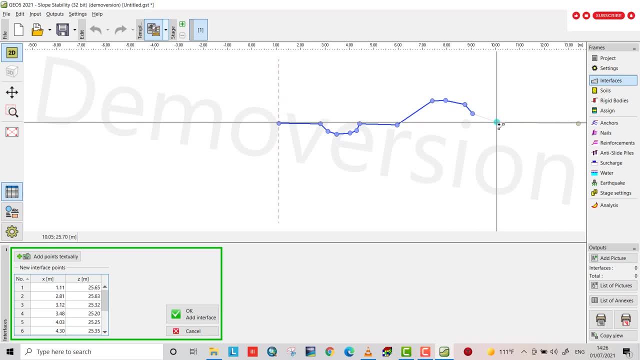 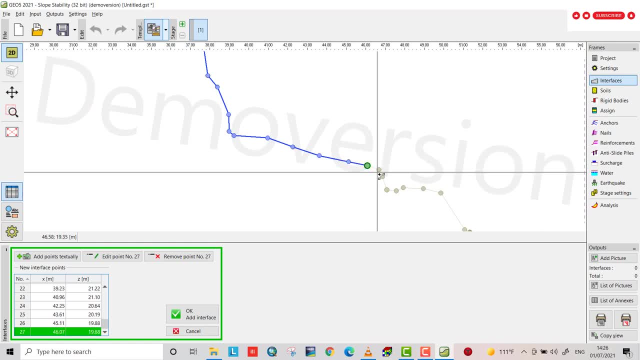 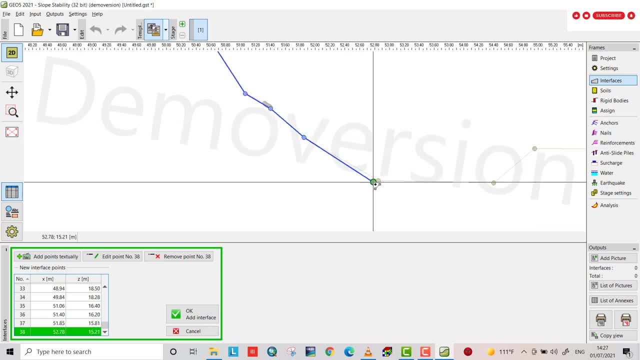 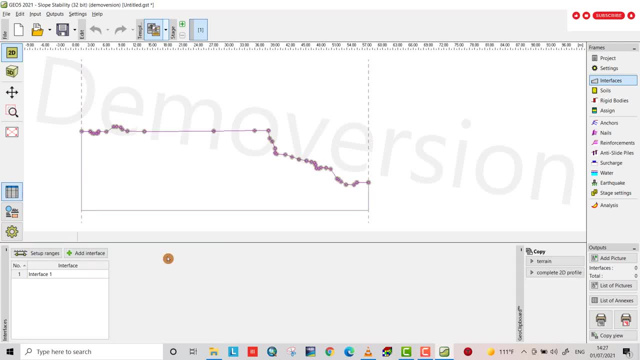 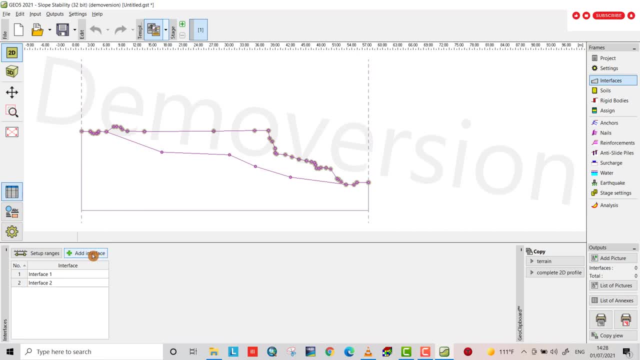 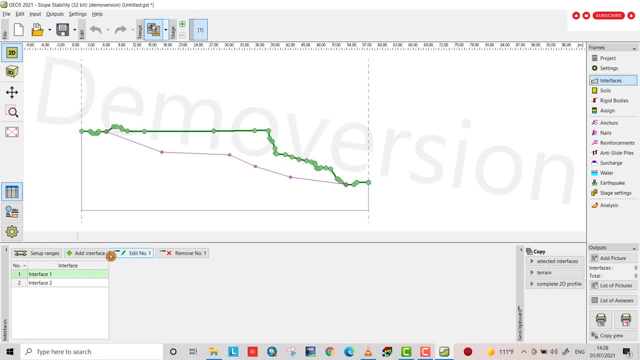 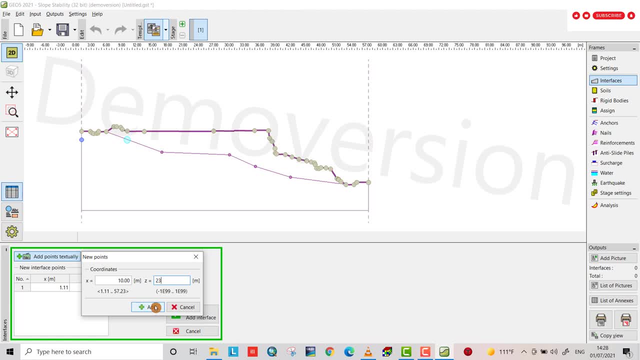 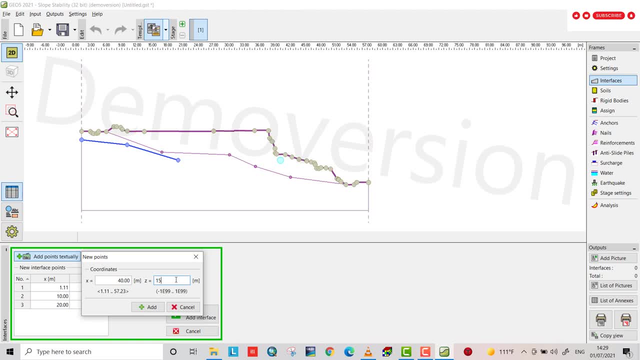 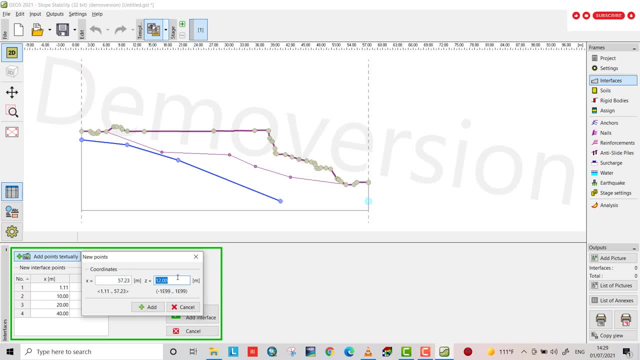 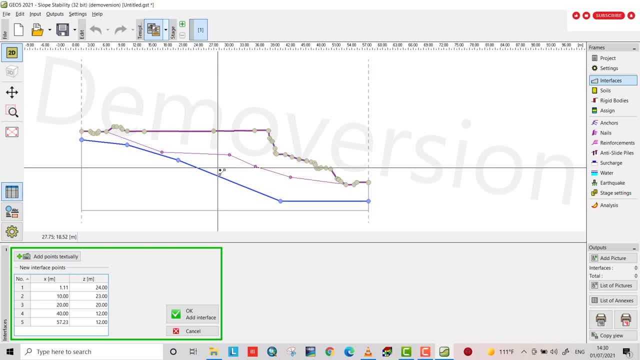 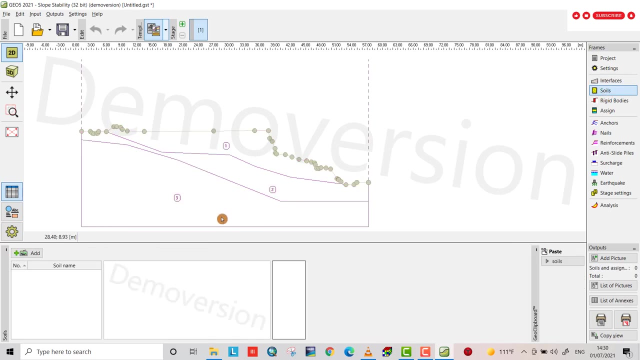 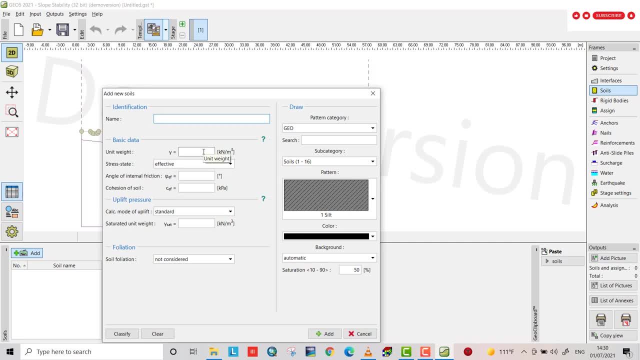 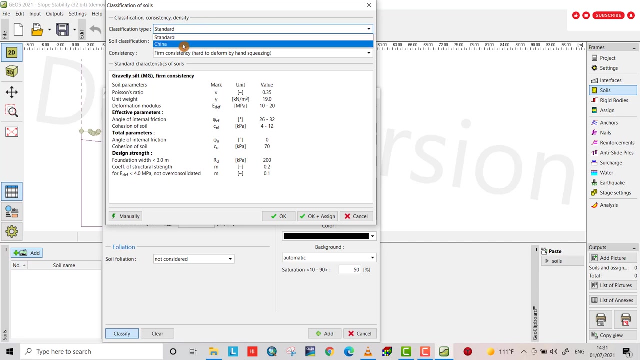 Okay, Okay, Okay. Okay, different types of soil. so if you want to define the soil by yourself, you can watch my video I put in, I put it in a description from classification. you see, we have from classification type, standard and China. I choose standard and that is a different type of soil. first soil I choose. 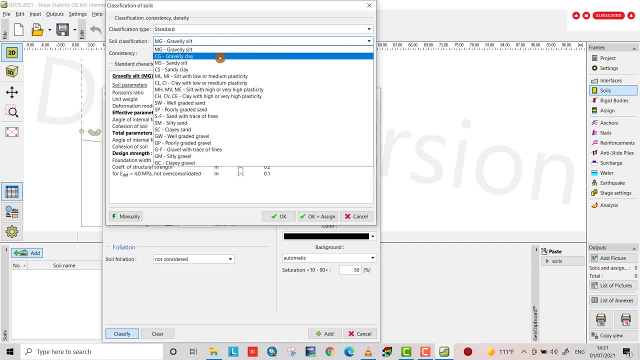 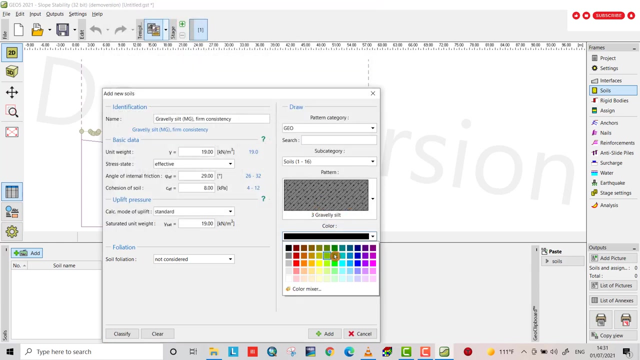 gravely sealed. gravely sealed, okay. roughly sealed, yes. and film consistency: I choose freedom consistency, okay. also, you can change the color, let's be green. you see, directly program fill all the gaps, you see. for angle of internal friction, there is already 23, 26 to 32, which is the 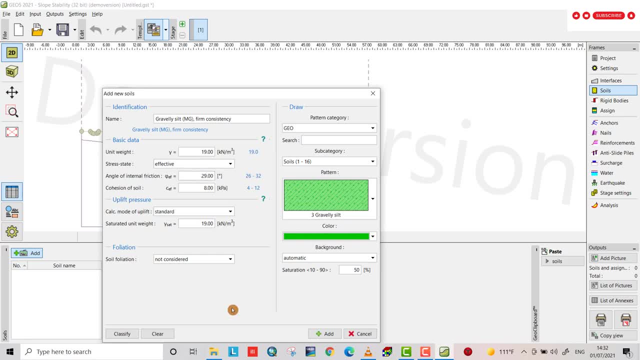 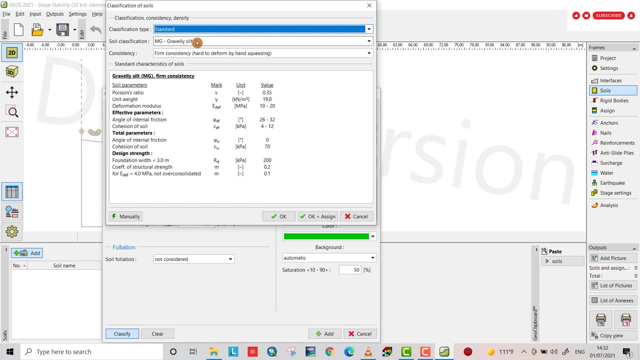 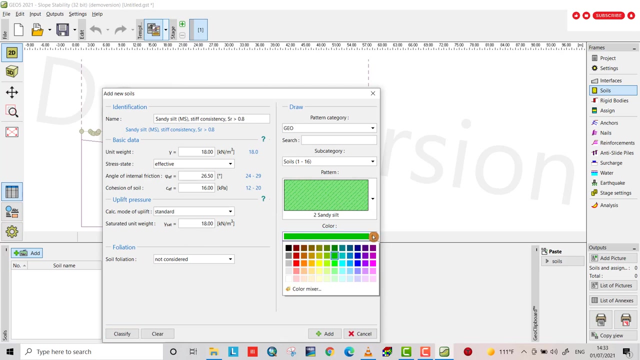 program. choose the 29. you can change the data. okay, another one, another one. I choose MLMI. I should sign this out. okay, let the film. consistency, Steve, consistency, consistency. okay, choose Steve. consistency, consistency. this data is obtained from labs or from literature is okay, and you can choose the color and change the color. let be this one. 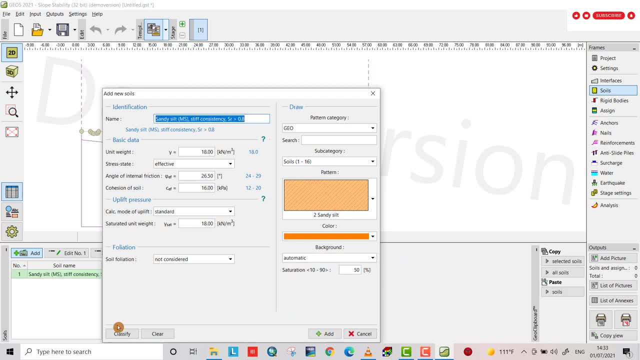 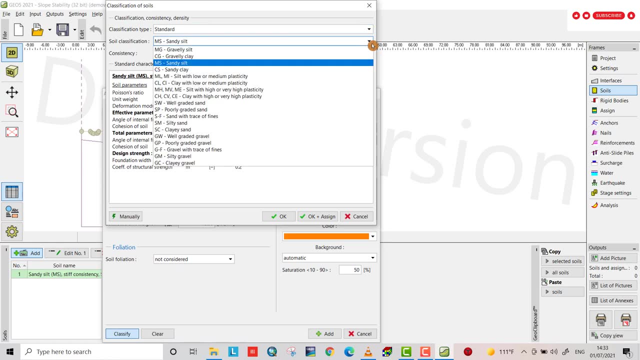 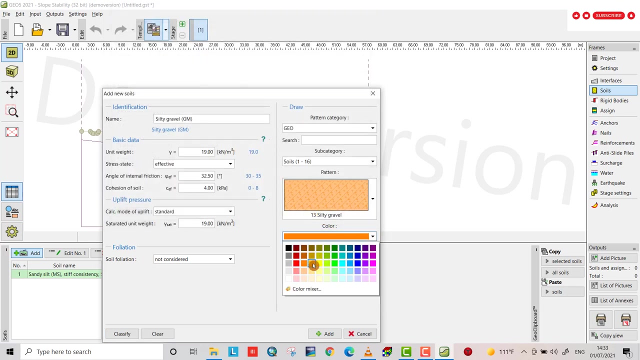 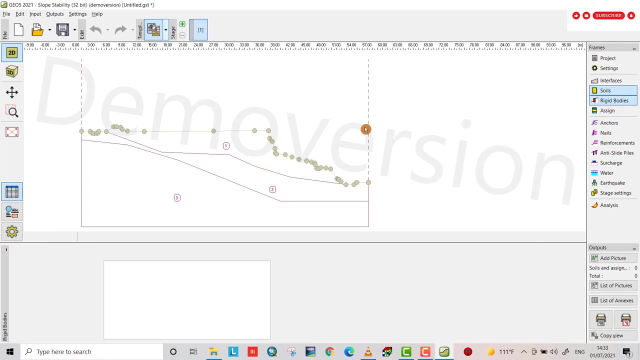 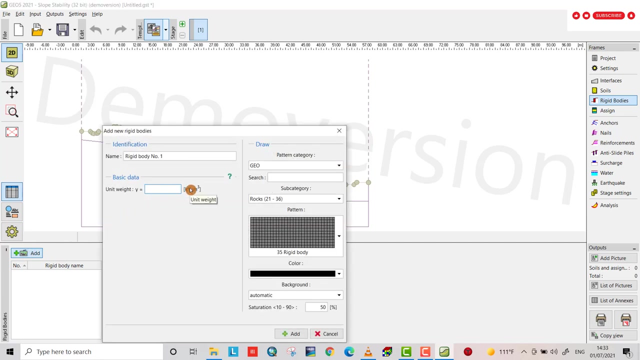 okay, another soil I choose still gravel, yes, medium-dense, okay, medium-dense, okay, and sign and change the color. it be this one. okay, now we have a different solace also. we can provide rigidbody. rigidbody- there is no change in the rigidbody, just provide the unit weight- let be 21 kilonewton- and the 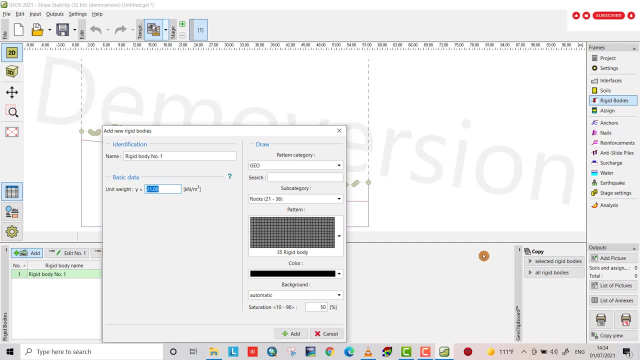 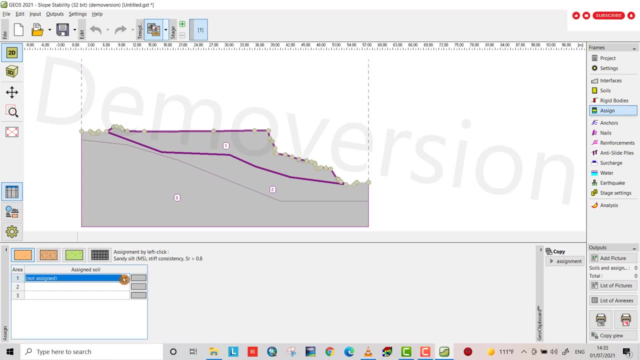 color: let be black. okay, now I'm going to assign for face layer. okay, now I'm going to assign for face layer. okay, now I'm going to assign for face layer. okay, okay, grub with it, yes. second, there recommend silky gravel and force it the layer you. 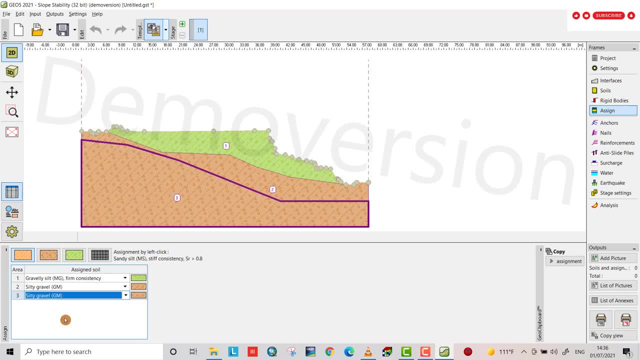 can feel: result: provides at Europe. let's change the color. now, still feel the gray color and force it to layer. you can still feel: provide silver. let's change the color. no silky gravel, no silky gravel, no silty gravel. you can see theAST grub: silcoat. 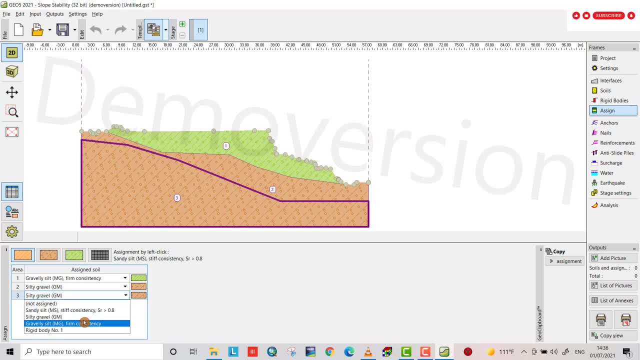 silky gravel, not this one gravel is still sandy here. okay, i don't provide a rigid body. if you have the rock bed, so you can provide rigid body, but i don't provide also on personalities and slides. third charge: in this stage i don't uh provide search. in the next stage, i provide. 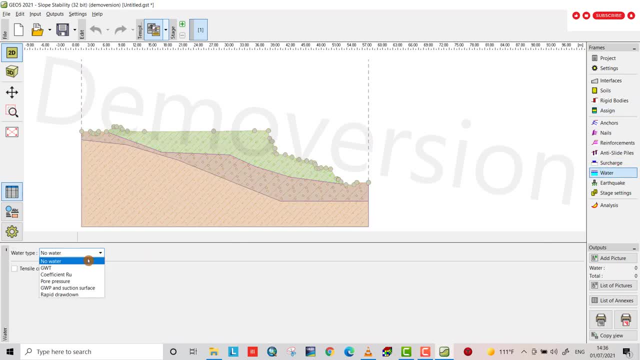 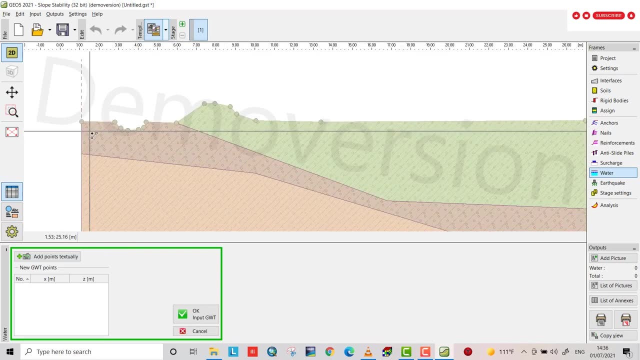 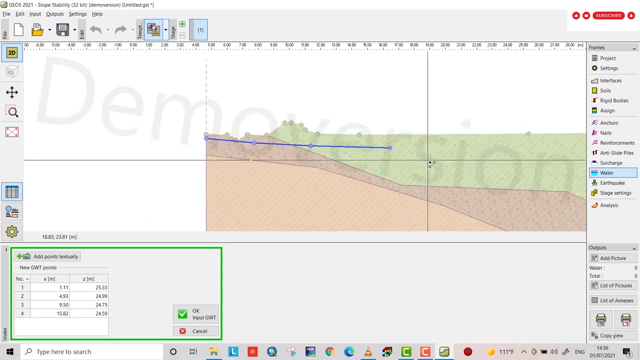 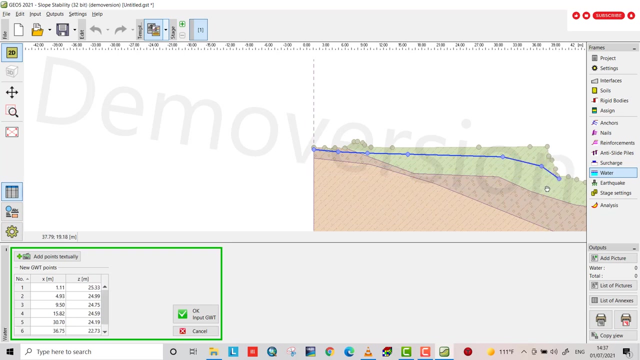 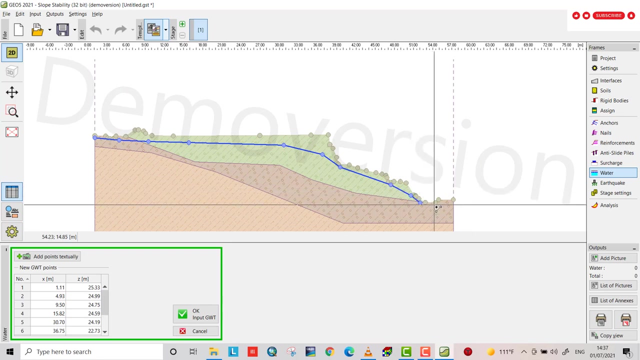 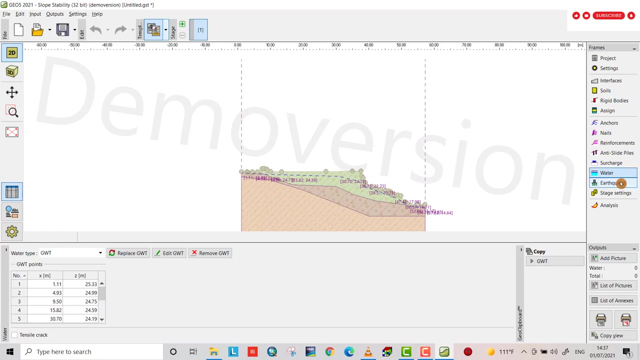 search. let's provide what table? okay, input ground. what table i draw? okay, earthquake you can provide us to analyze this way, i don't use this. let's analyze bishop standard and also input graphically. i want, if you want, to find the slope stability for this section. 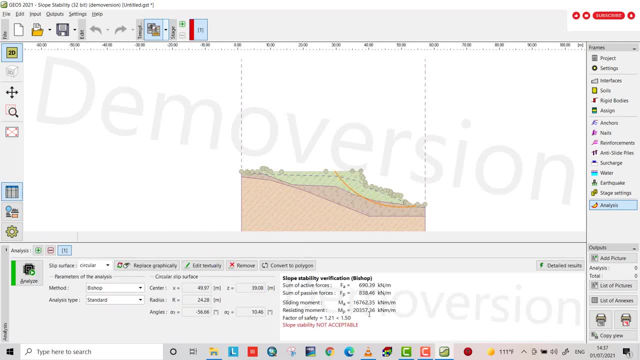 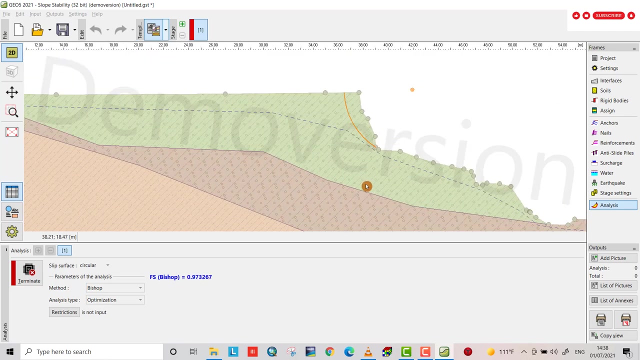 okay, analyze, you see it's not acceptable. 1.21 smaller than a limit is the limit. also, you can optimize to find the most weak slides. just use optimization. you see how the program optimize and find the weakest slides. you see that is the weakest uh slip surface, which is 0.97. okay. 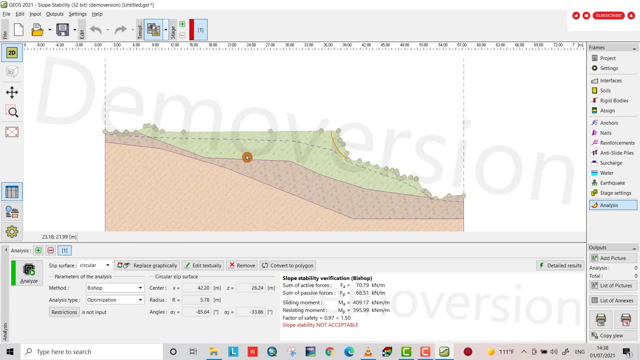 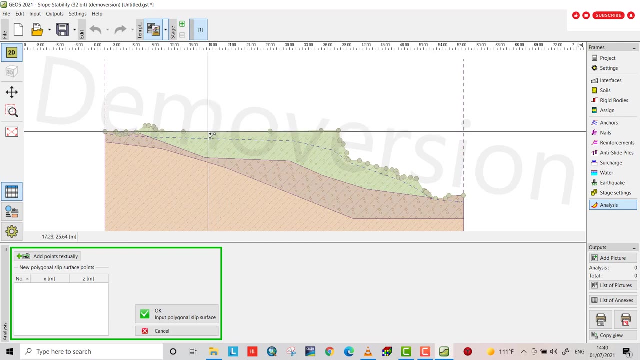 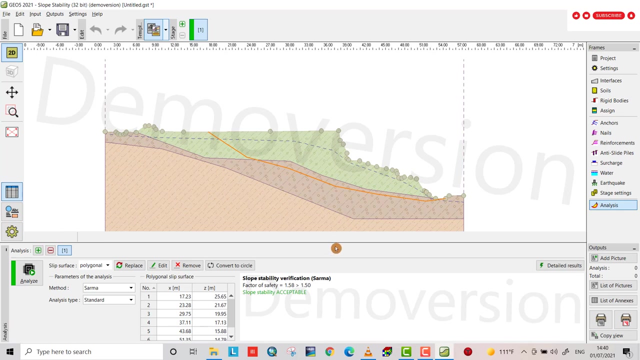 also, if you have a weak layer, you can find the slope stability or factor safety for this slice by, not by circular, by polygon. if we, if we check the uh stability of this section okay, analyze, it is over the limit, so it is uh safe also. it is. 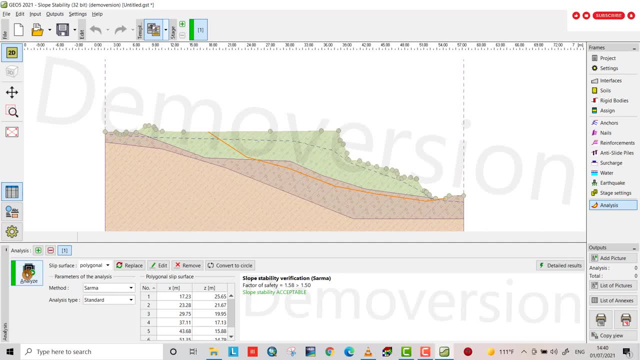 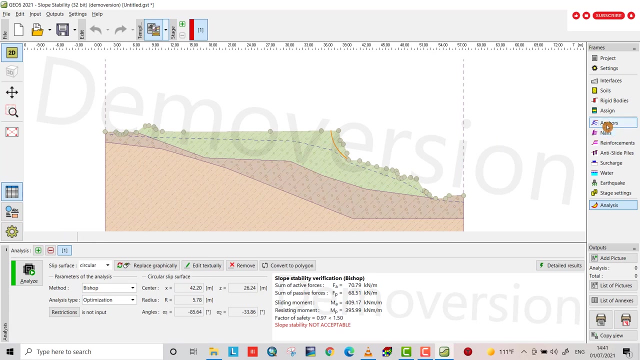 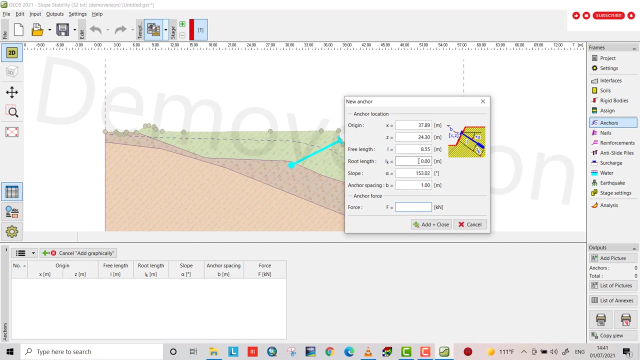 find some solution for this slope. stability for the stability, sorry, yes, not circular optimization provide, no, no, just analyze, cancel, just analyze. the surface is not safe, so let's provide some solution. we have anchors. let us provide anchor graphically. you can also use the any of the 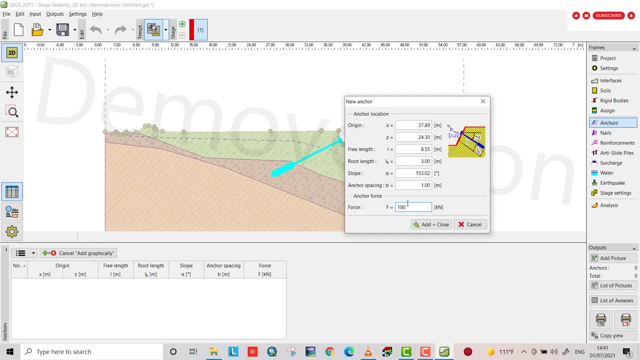 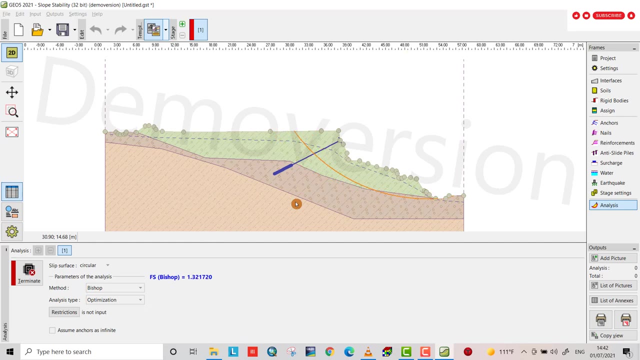 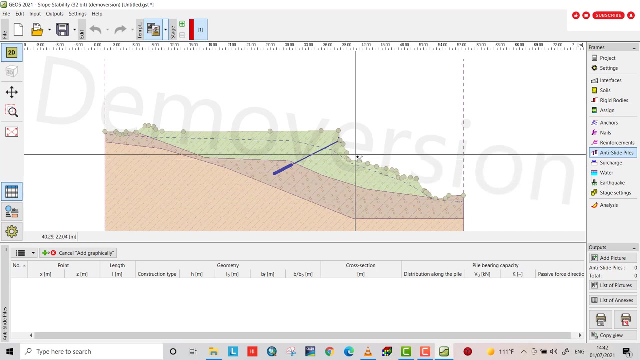 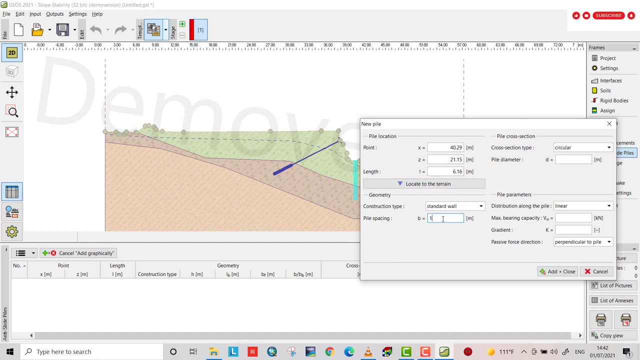 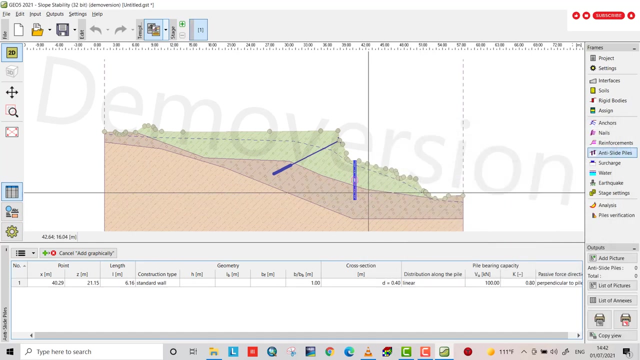 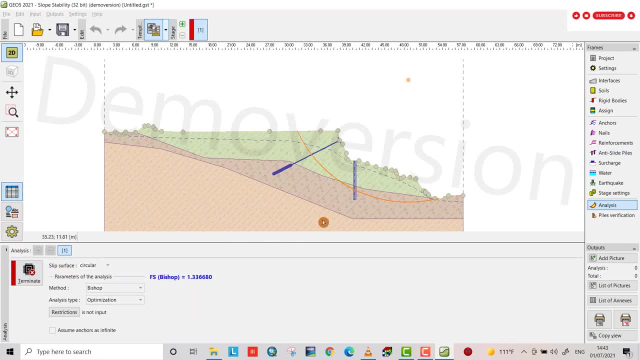 i mean it's. you can't see any difference. let's analyze any it's. you can't see any difference. let's analyze any it's. you can't see any difference. you see it's 1.27. you see it's 1.27. change it to. 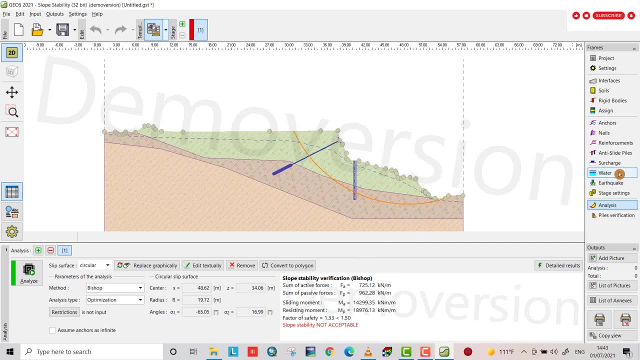 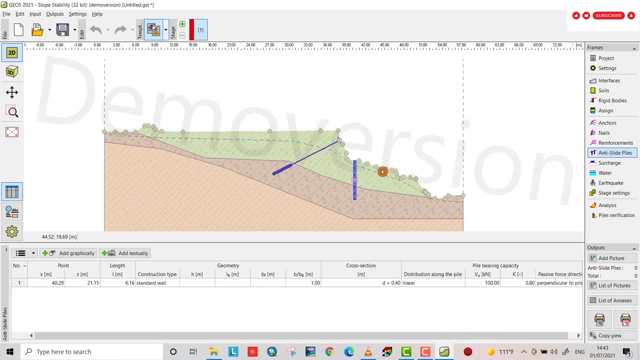 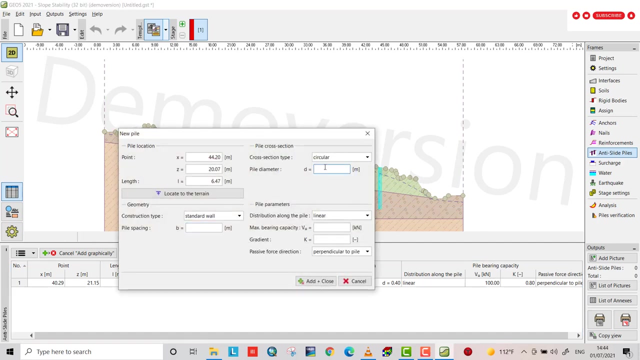 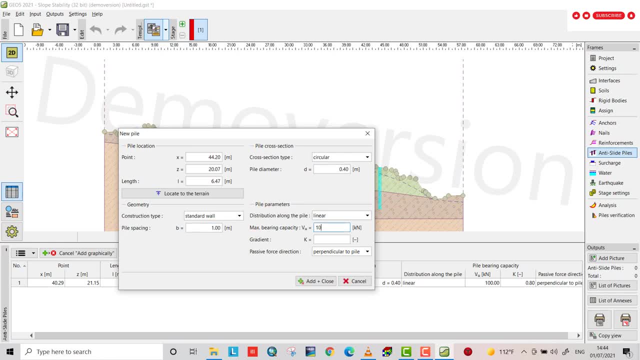 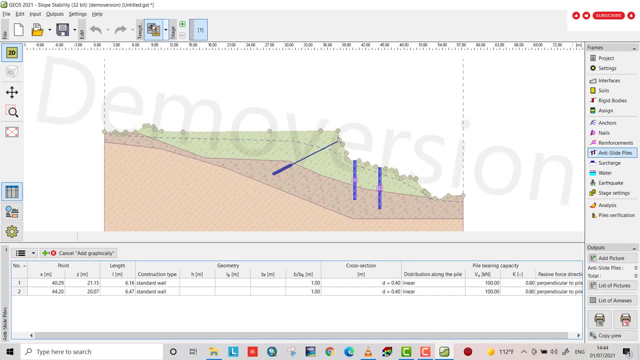 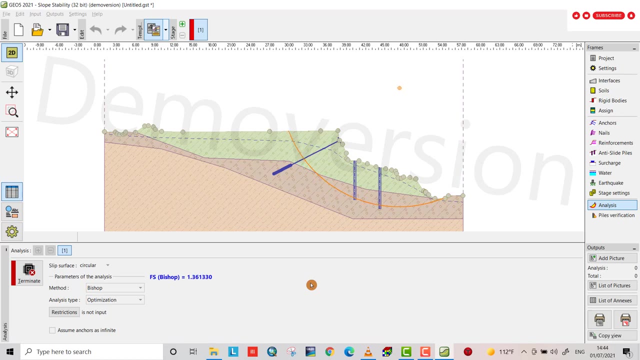 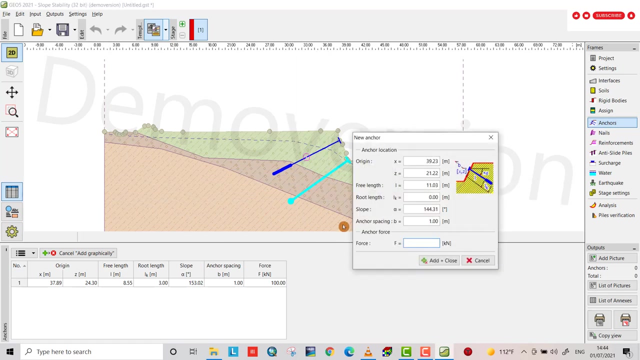 d 0.4 b1 meter d 0.4 b1 meter d 0.4 b1 meter. 100 0.8, 100 0.8. okay, analyze, analyze, analyze, analyze, analyze, analyze, it is still not safe. 1.35 is not safe. so what should? we can do, we can provide another anchors. 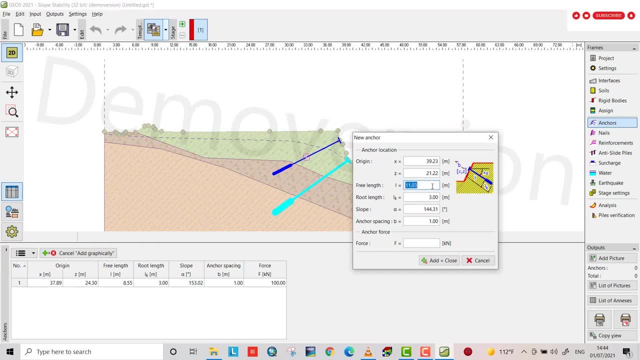 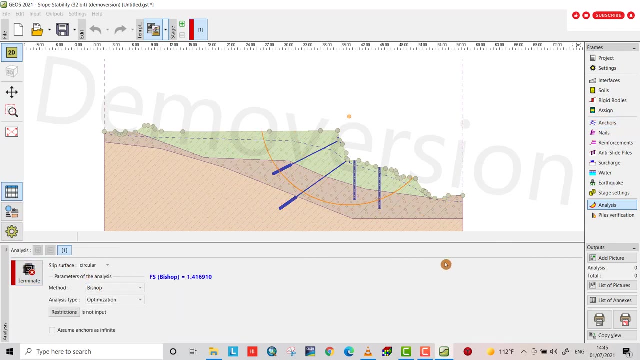 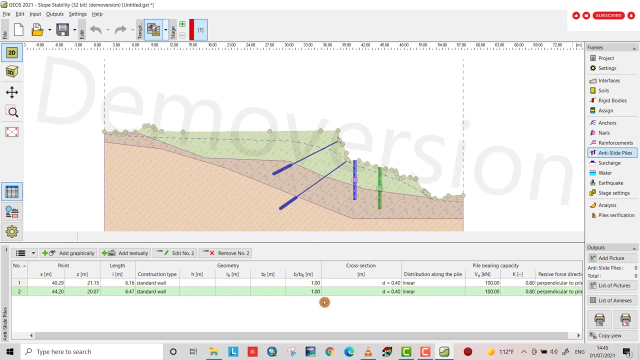 perimeter and it became 100 kilonewton. okay, this time analyze 1.42: it is near to the limit, so you can provide another anchor. or change, sorry, or change is the length. is if 1.42 it is near to the limit so you can provide another anchor. 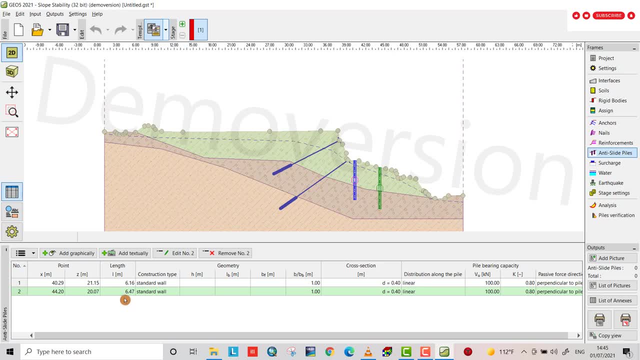 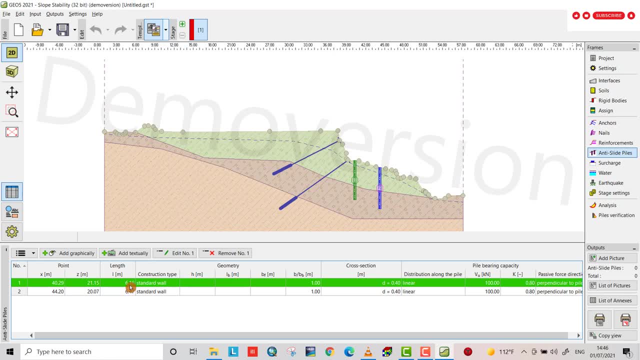 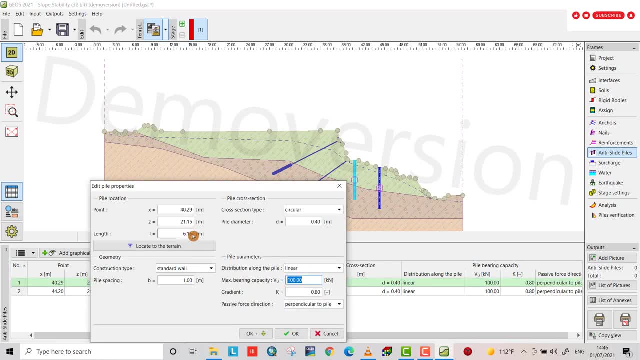 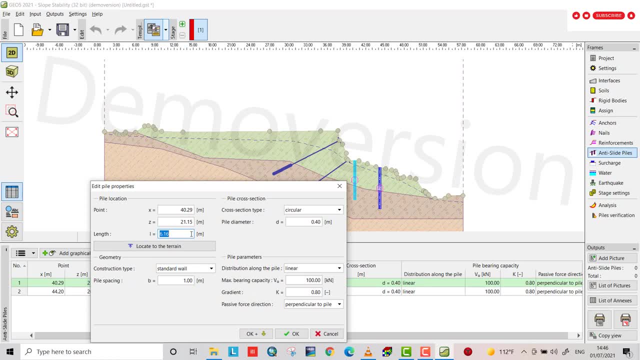 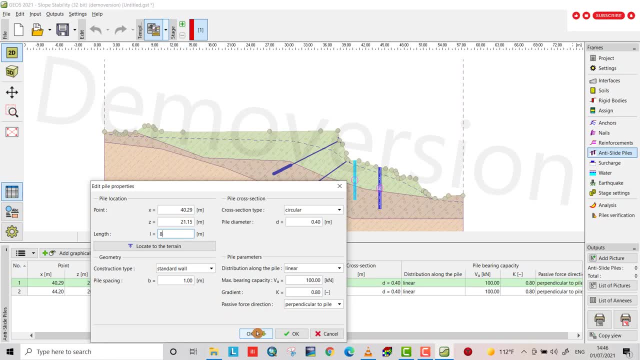 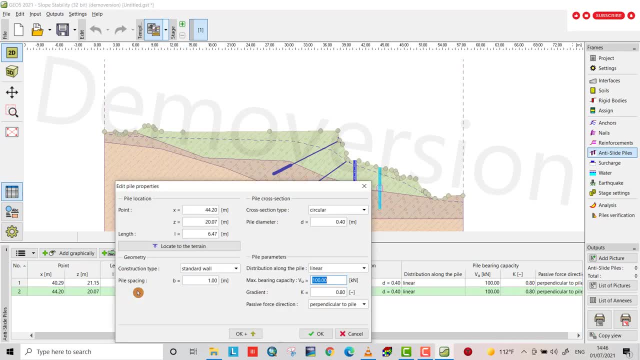 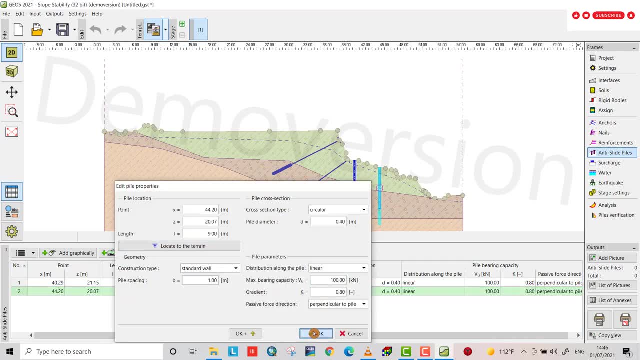 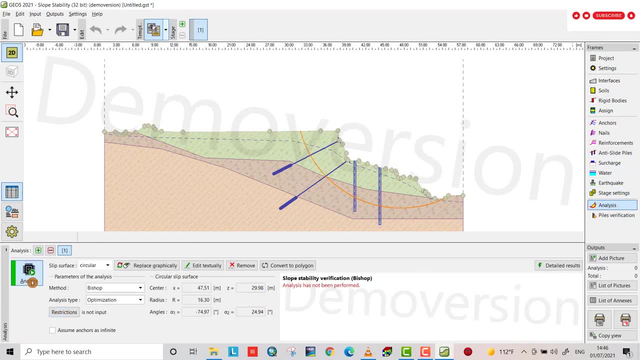 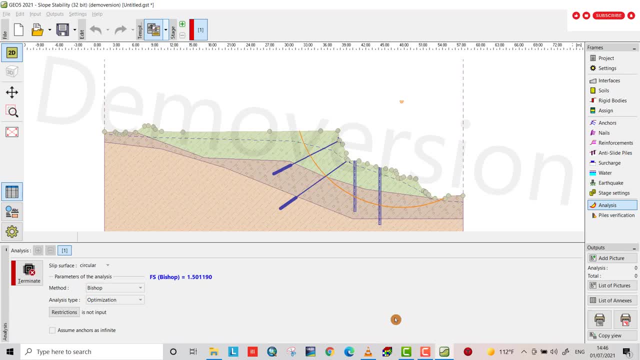 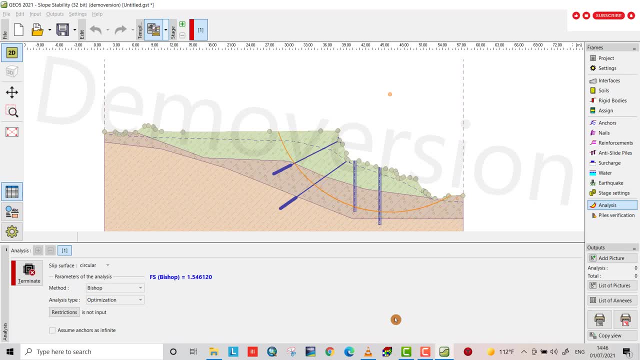 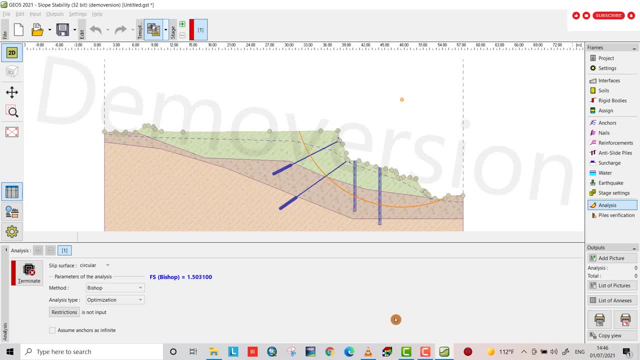 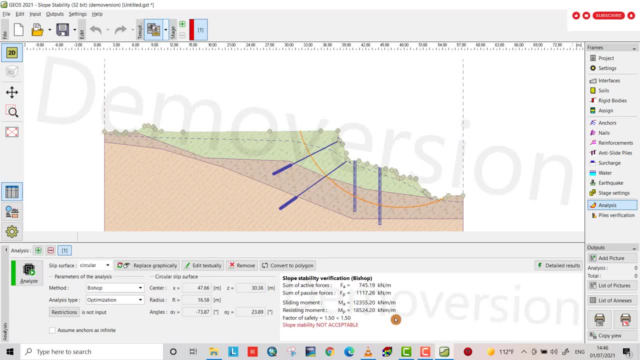 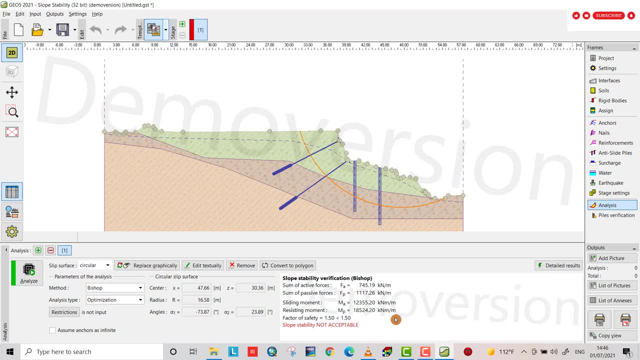 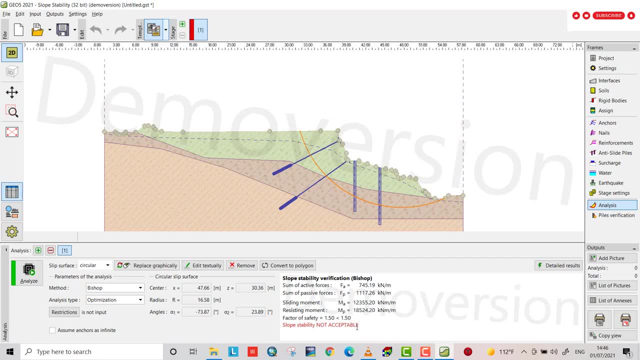 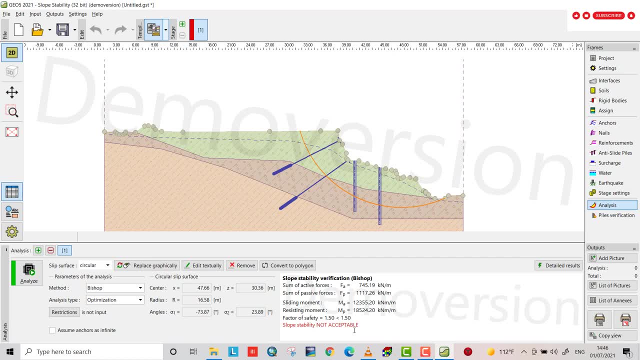 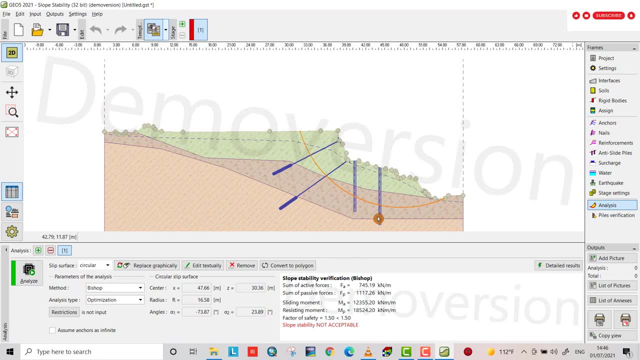 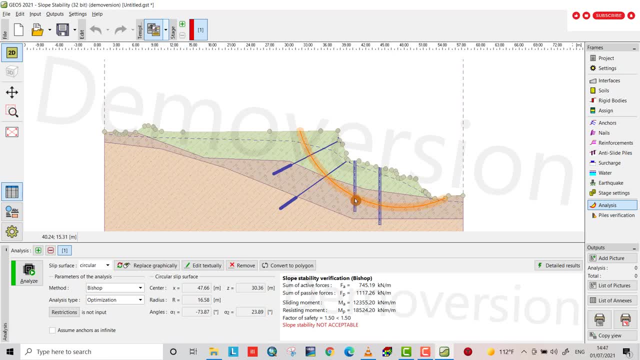 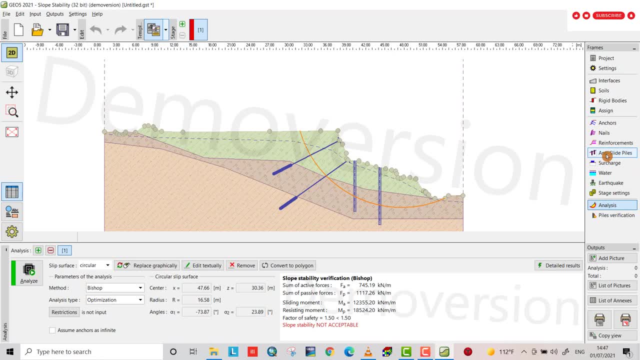 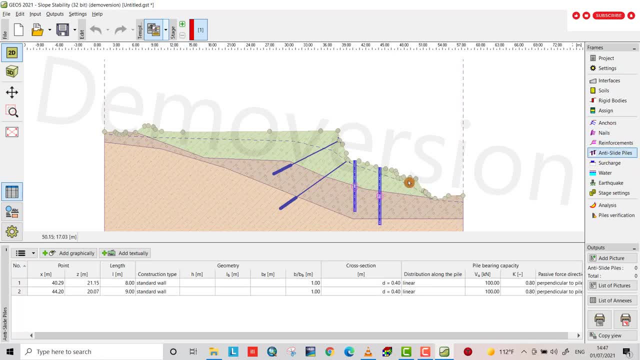 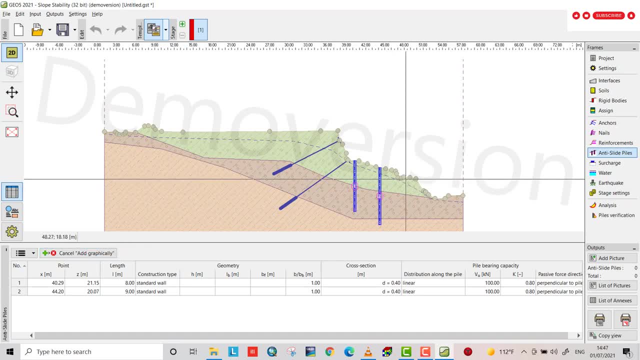 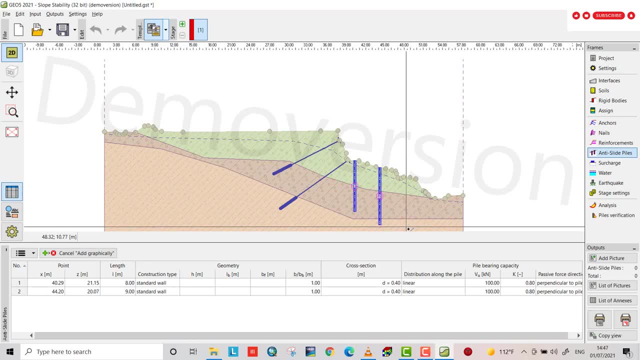 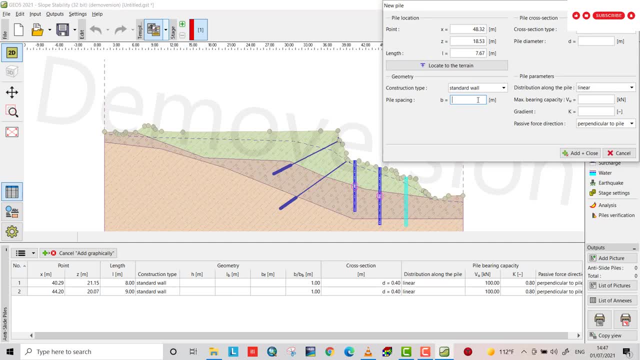 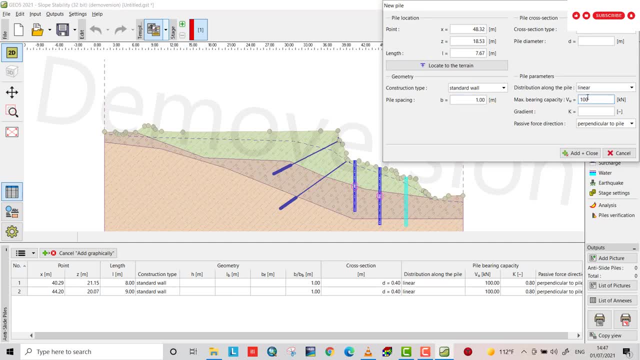 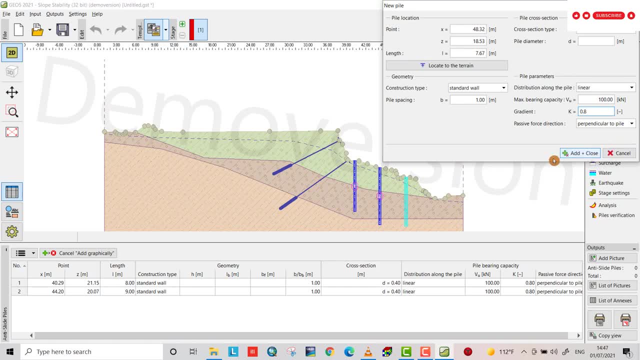 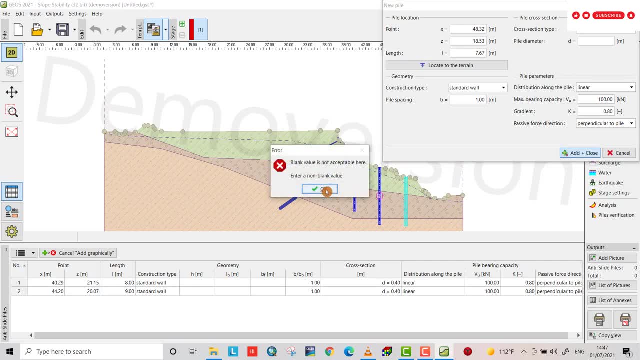 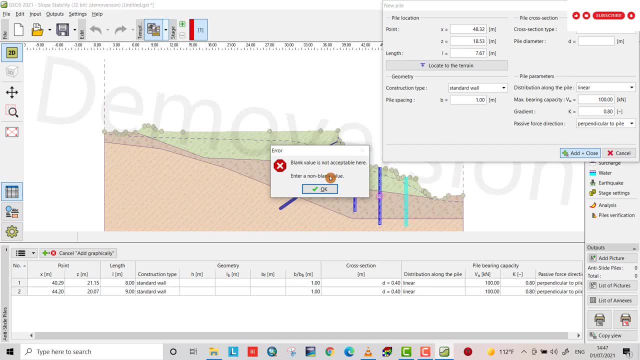 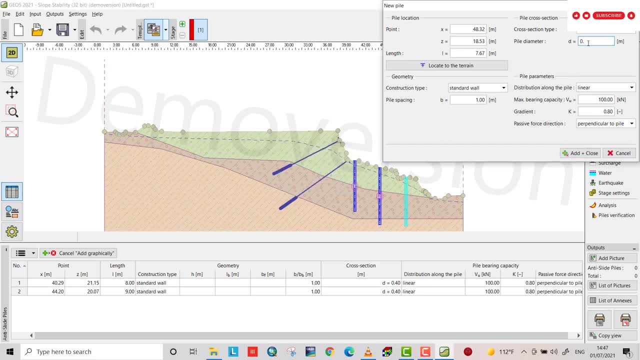 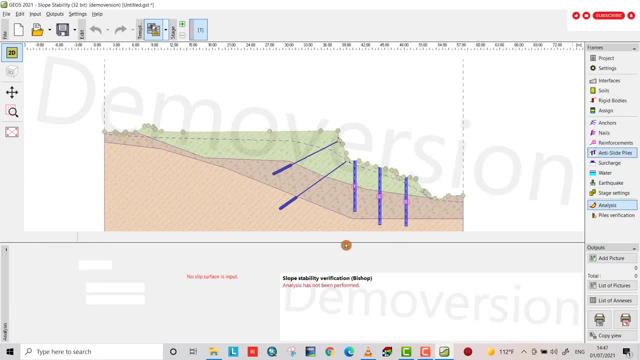 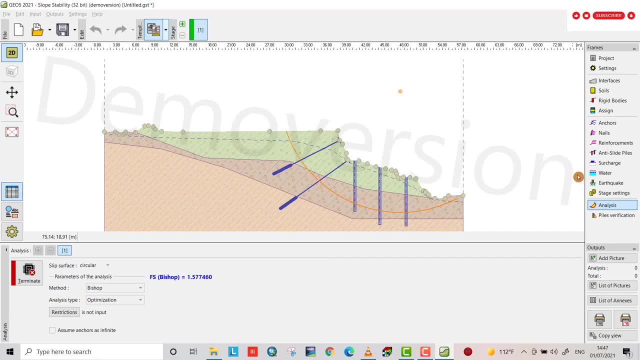 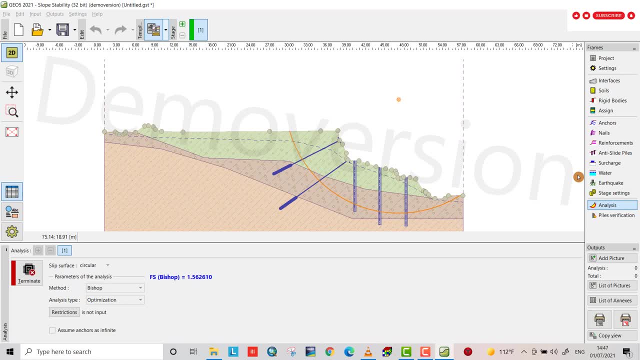 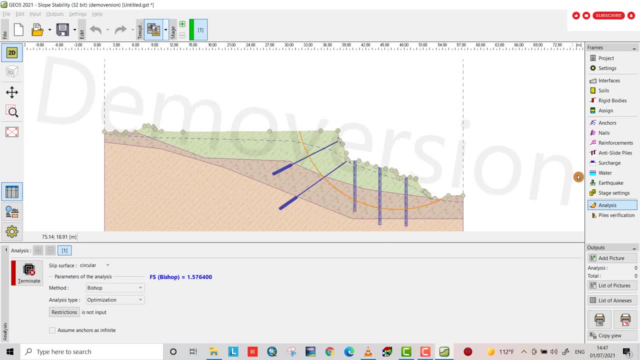 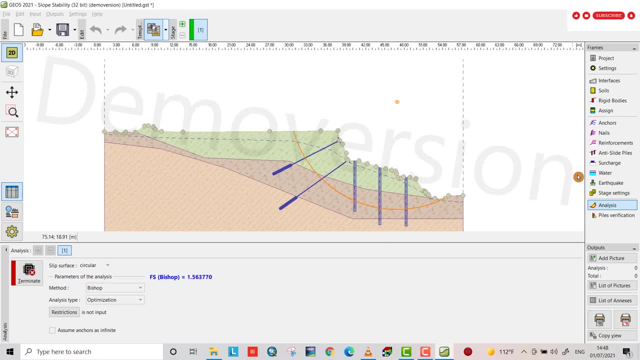 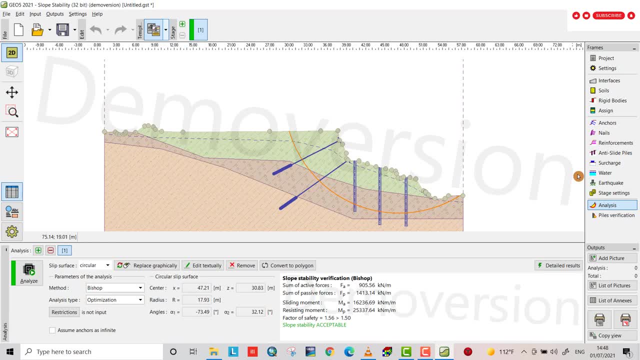 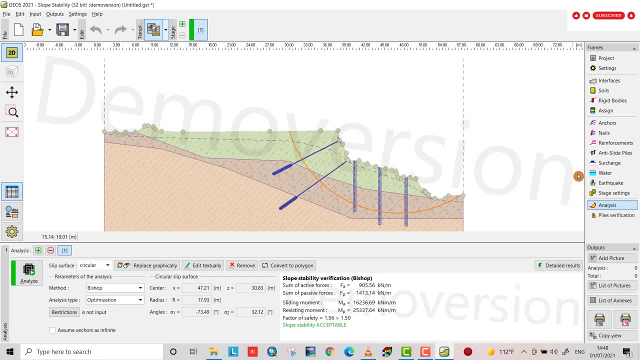 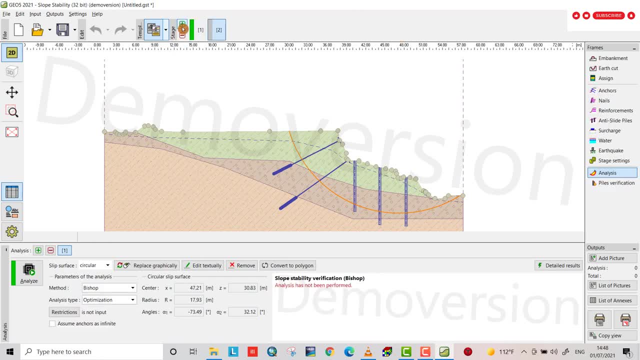 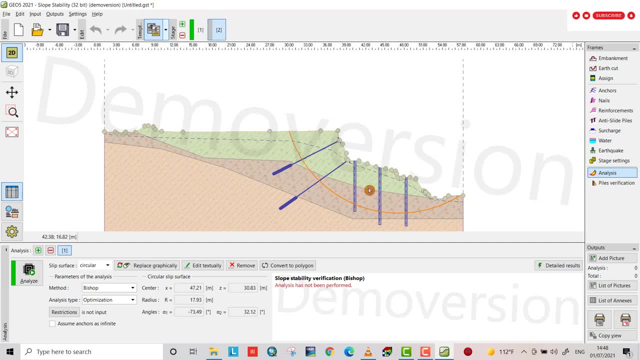 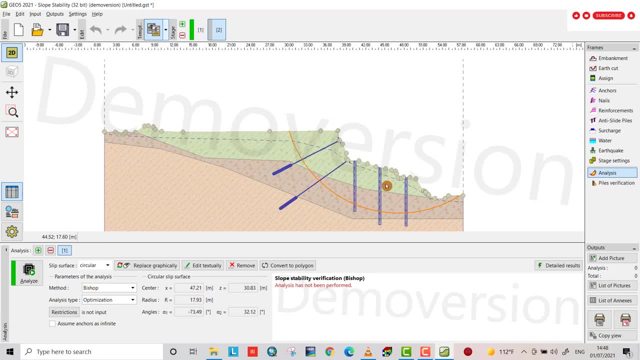 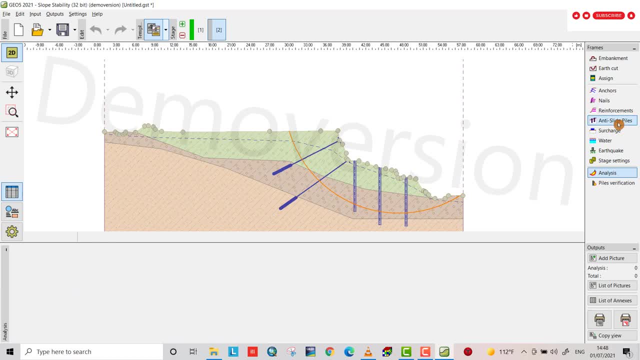 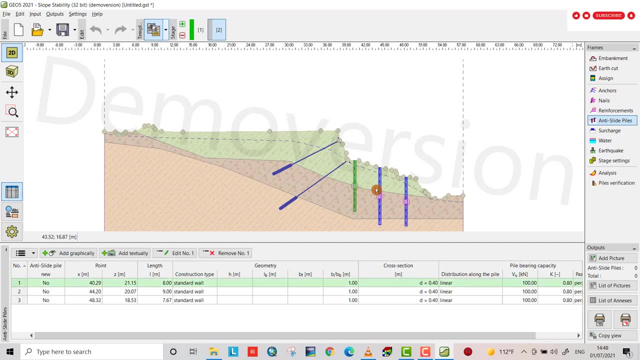 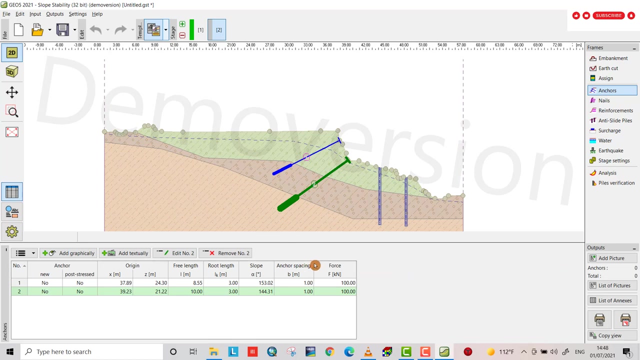 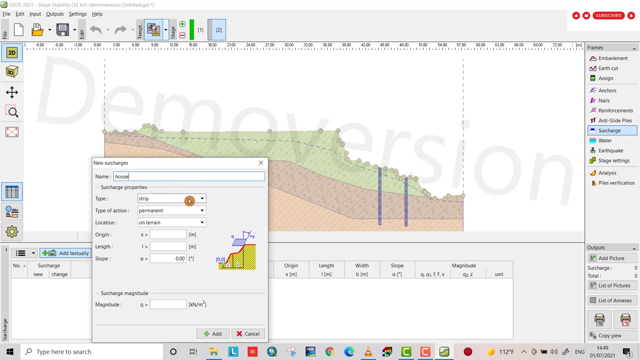 or change. sorry, or change is the length is. if anti or anti-slide virus: okay, I remove this. yes, I don't need this one. sorry, anchors: yes, remove also. I try. I want to provide search charge a textually: house, for example, we have a house strip: yes, permanent. 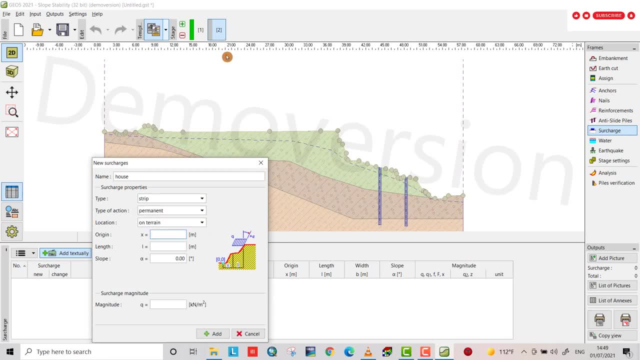 on-terrain X, from where, if we have here from 21, from 24, okay, from 24, and language, is it be 6 meters or 8 meter? sorry, 8 meter alpha, okay, and the magnitude did be 100 kilo Newton per meter square. 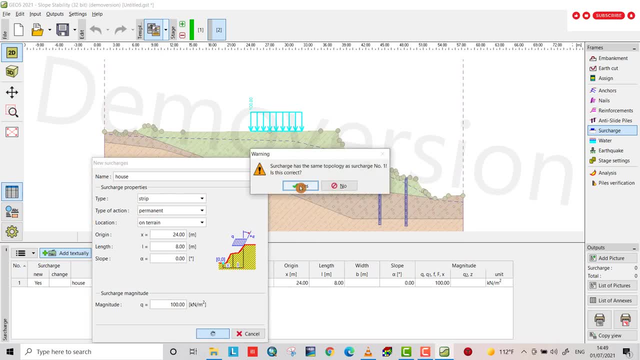 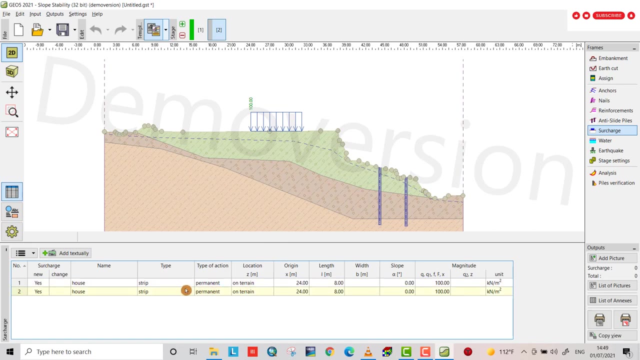 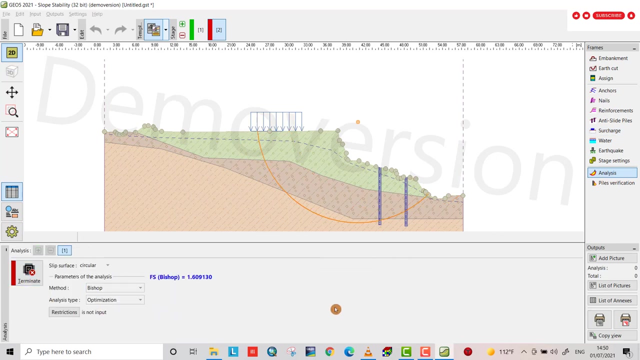 yes, yes, no one, we need one. we move. yes, let's analyze a iodized is the stop, the ability? you see one, a stop, stability is not acceptable. one, one point, twenty one. also, you can provide anchors and find the solution for the slope stability, if let's, if we provide anchor. 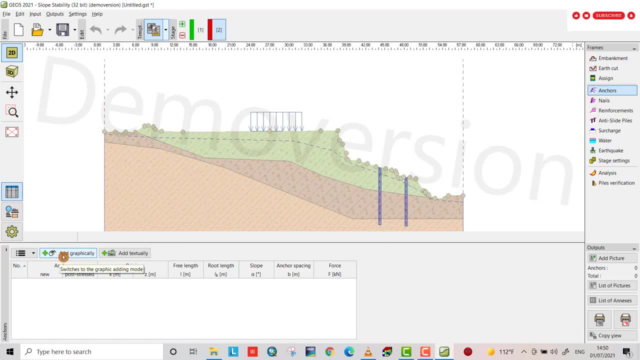 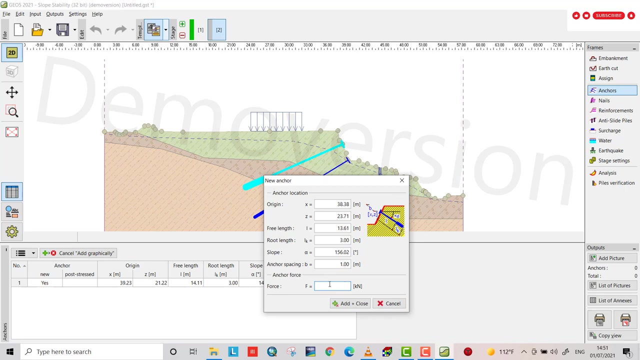 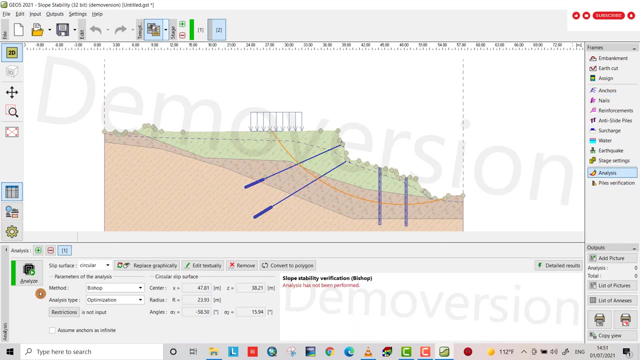 here three one hundred, okay. another anchor here: three one hundred, okay. analyze 1.33. also, you can provide a retaining wall. I just want want you how you analyze the slope stability and in the next tutorial I find a solution by providing a retaining wall for just for the stoppers. I hope it be helpful. have a nice time. you.